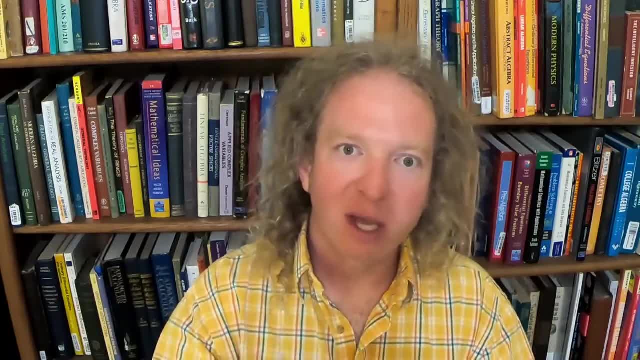 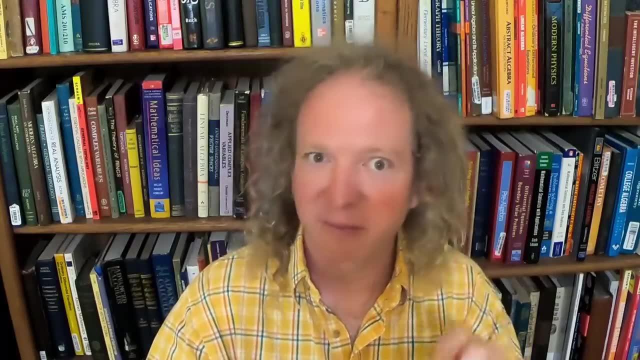 In this video I want to talk about one thing that you can do that is going to make you do better on your math test. This is something that you can do that will help you get A's in math on your math test. It's just one thing. 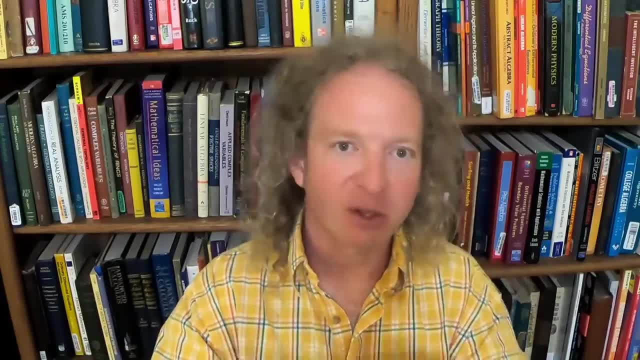 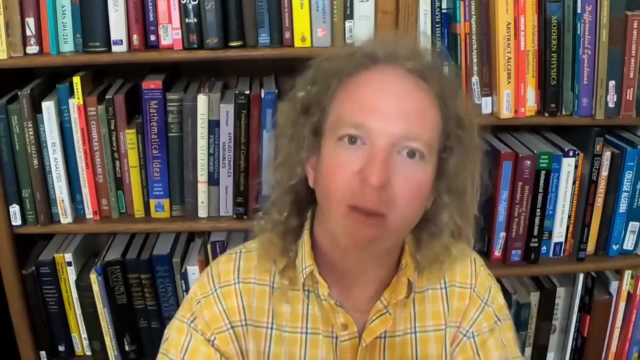 So, of course, for every test, you study, you do the homework, you go over the notes. If there's video lectures, you watch those again. I mean, you do your best. You're probably doing at this point everything you can do. 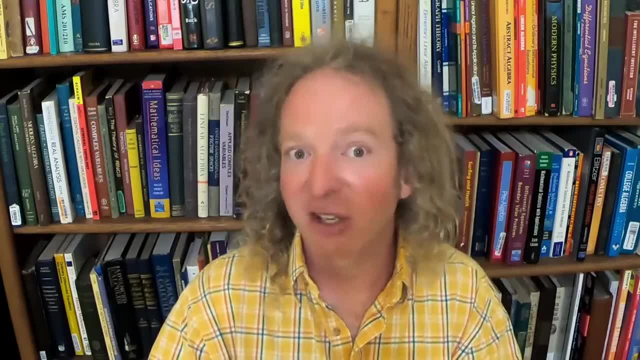 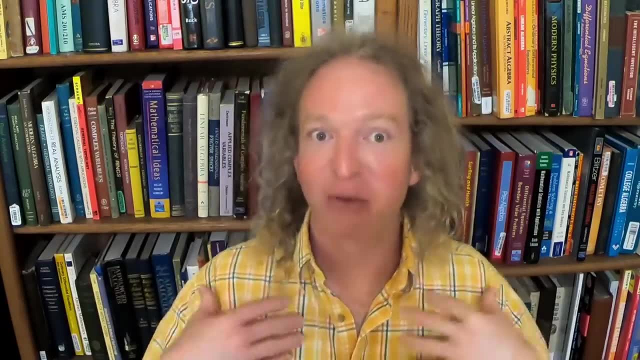 But there's one thing that you might not be doing, And I actually met someone else recently- well, not that recently, maybe a few years ago- who actually does this, And I was actually quite impressed because I thought I was the only person in the world who did this. 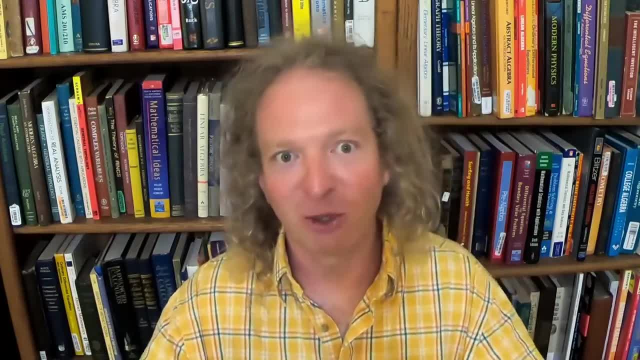 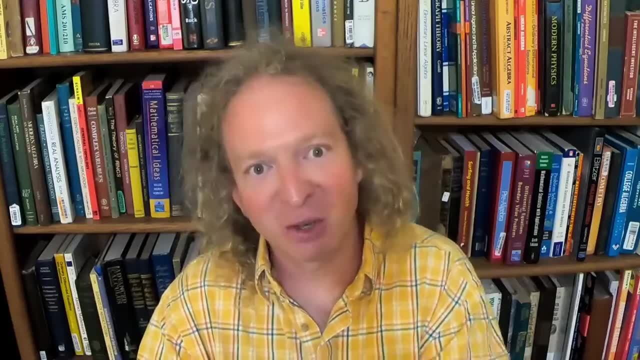 I mean, maybe that's a really dumb way to think, like I'm the only one who's doing it. I mean, I did this on my own, I came up with this strategy on my own, And so to find someone else that's doing this, I think is interesting. 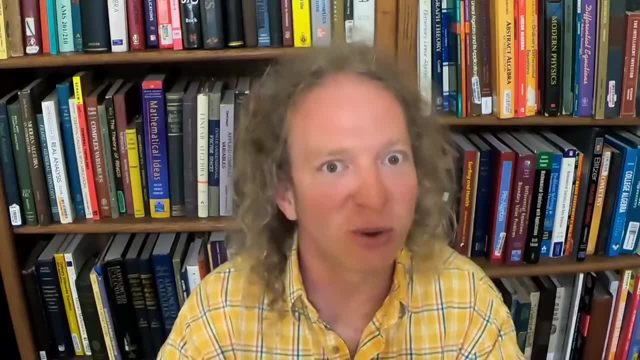 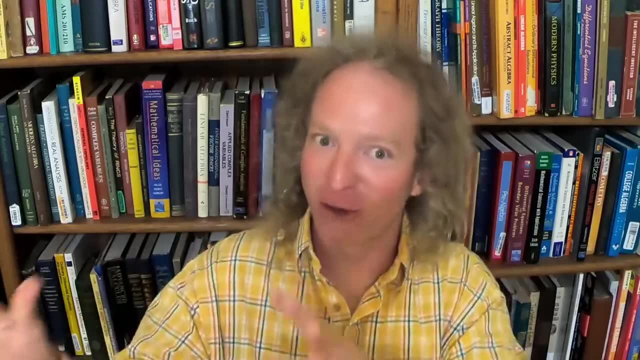 But it really does make sense. So what is it? What is this thing that you can do that will make you so much better at math? So it's speed, And I don't mean like drugs or anything but speed. 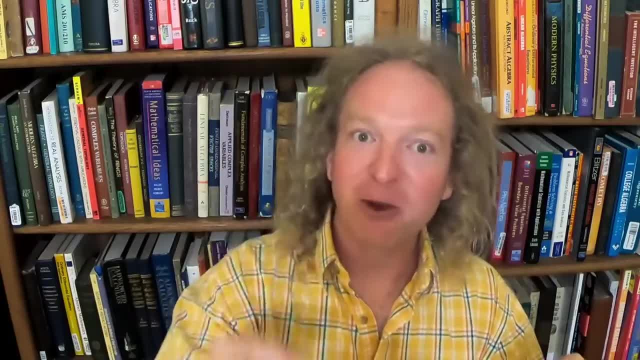 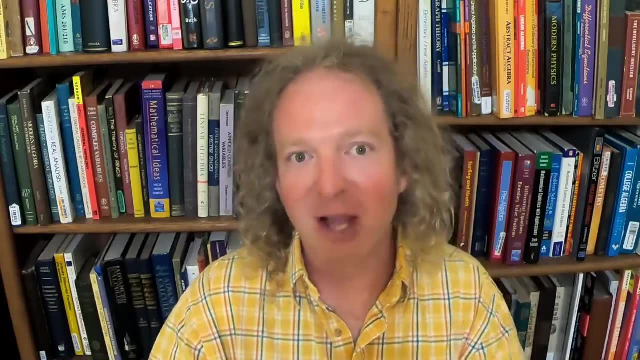 I don't know why I said that Speed. Speed will make you better at math, And you know. if you don't think speed is important, let me just give you a really weird example. When I was in grad school, I was taking a class. 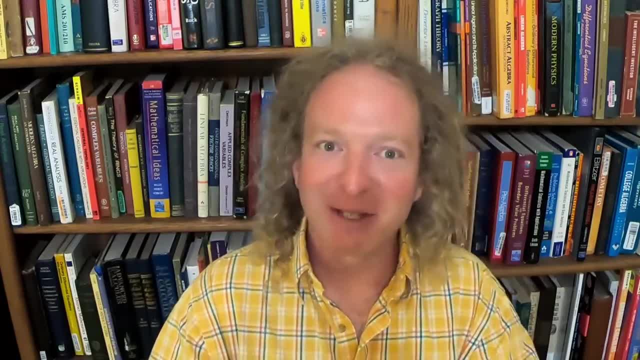 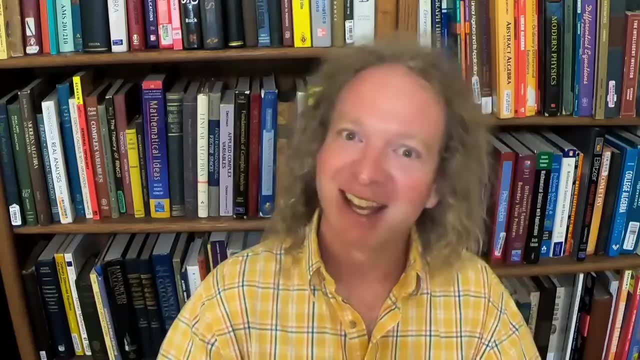 I won't mention the class. I won't mention anything about the class. Let me just say the teacher stood up in front and said: Speed is important. Just like they had this thick accent And he said it In a really angry way. 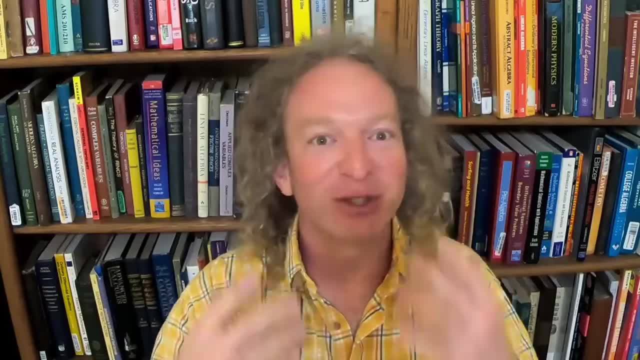 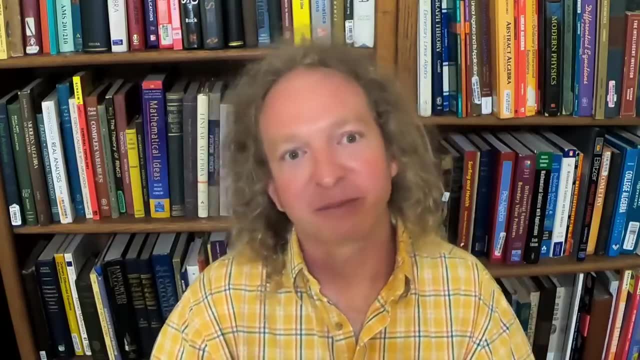 And I was like, oh, I was terrified Because I was struggling And I was so lost. I'm like speed. I can't even do the problem slowly. Why is speed important? You know, And he was right, Speed is important. 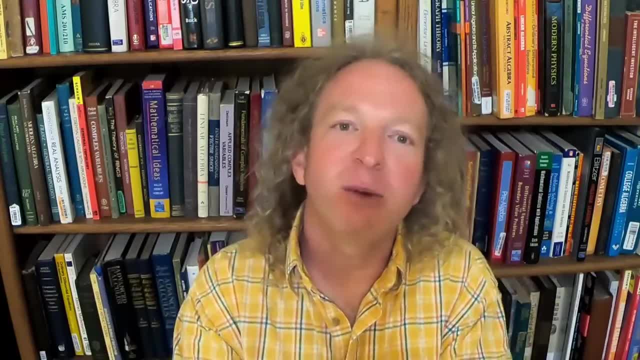 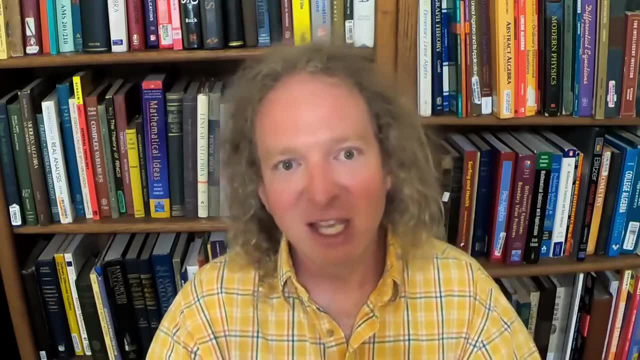 So what do I mean by speed? Well, by speed I mean you need to be able to do problems fast. Okay, It's important. I had a friend in grad school and he was really slow. He was really slow at math. 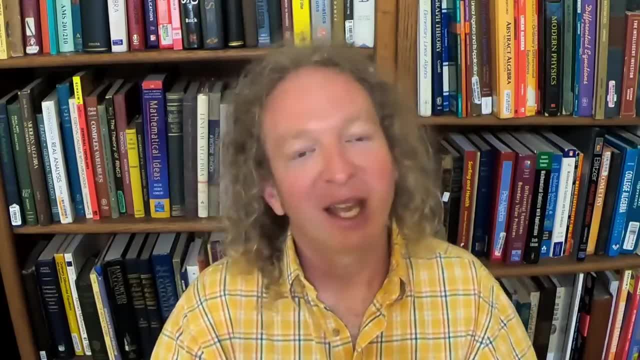 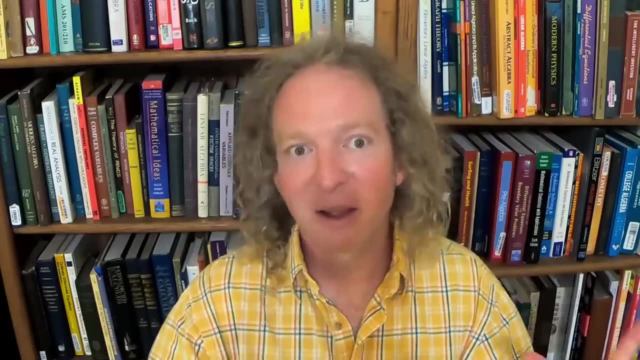 He just wasn't fast, But he was really smart And you know he took a class and he failed. you know a few of the tests, But he was able to come back and do awesome in the class by improving his speed. 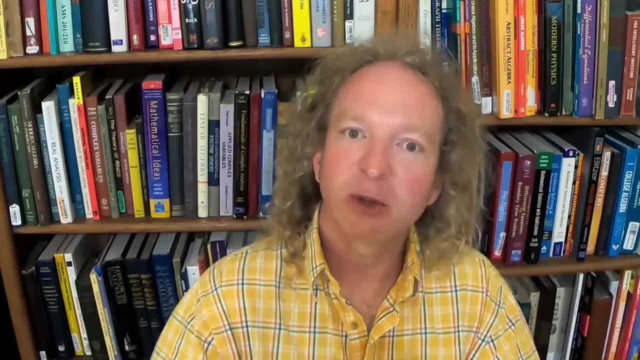 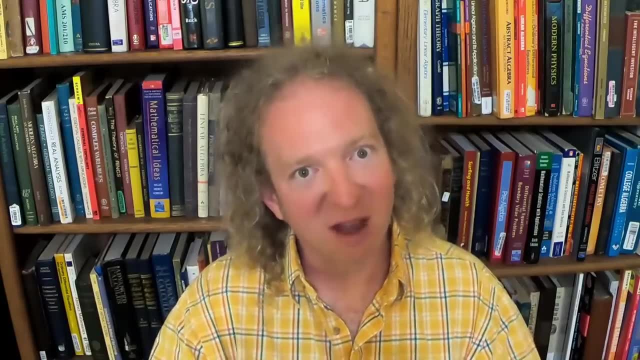 You might say: why did he fail the test if he wasn't? if he was so smart, It's because he was slow. He was really good at math, but he wrote slow, He thought slow. He was like the most chill dude you have ever met. 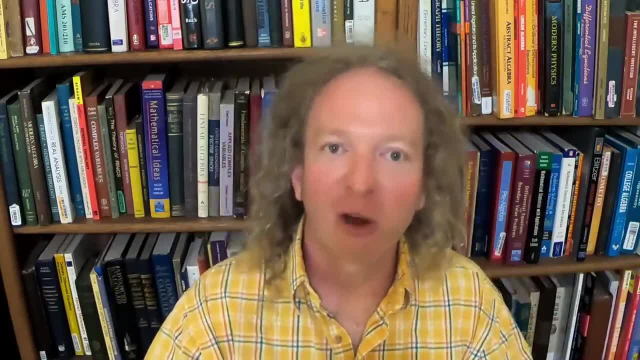 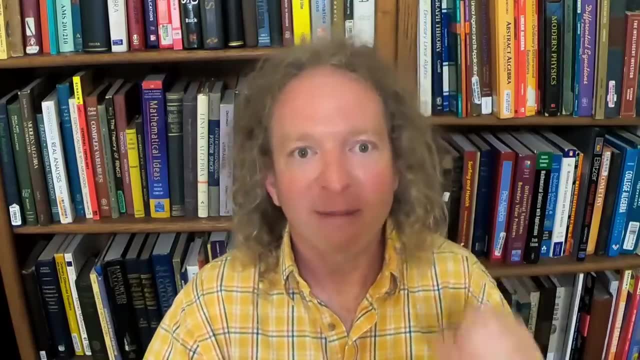 And he was brilliant, but he was slow, So he trained himself to work on speed. So how do you do that? Well, you want to do the problems fast, Okay? So after you've studied and done everything you can do for your class, you want to work on speed. 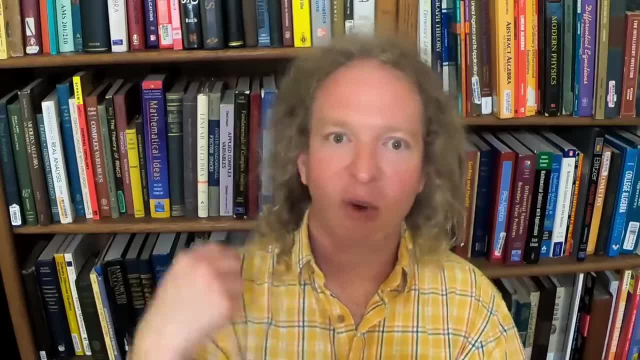 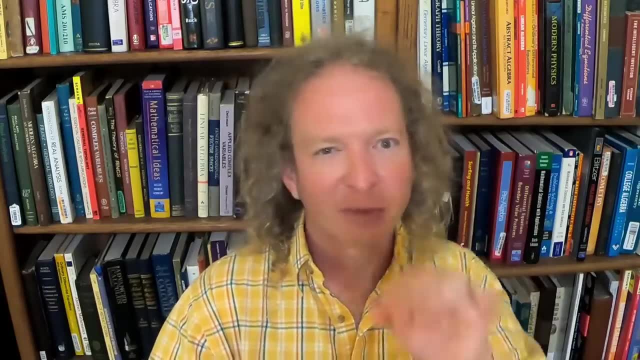 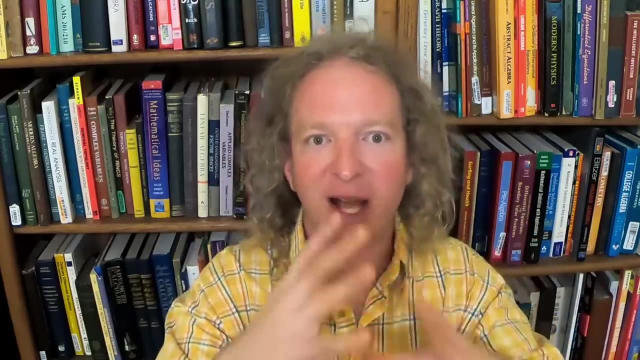 You want to work on like doing problems quickly and correctly and just speed, And this is something that I always did From the very first math class I took in college, which was the class before intermediate algebra. I took this intermediate algebra developmental math type class and then I took college algebra. 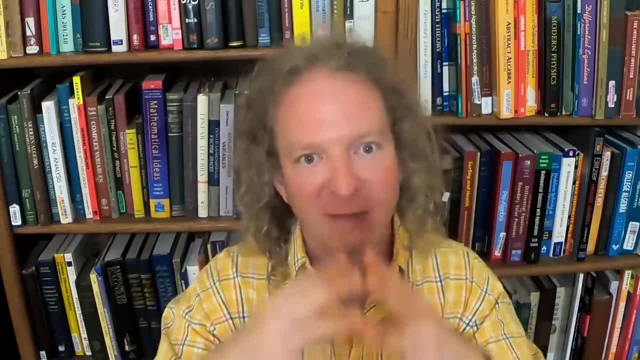 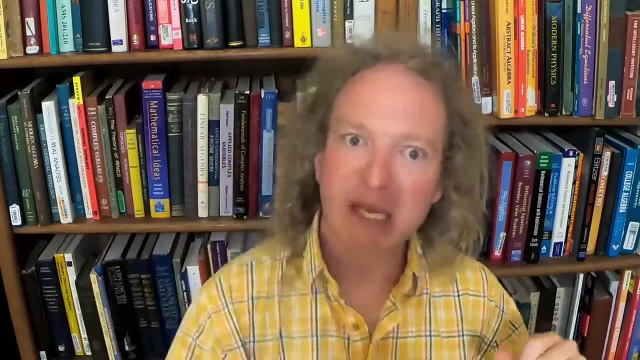 I mean, I started from the very, very beginning like rock bottom of math in college And even from then I remember sitting at the kitchen table working on speed. I would work on being fast And the reason is I had this huge fear. 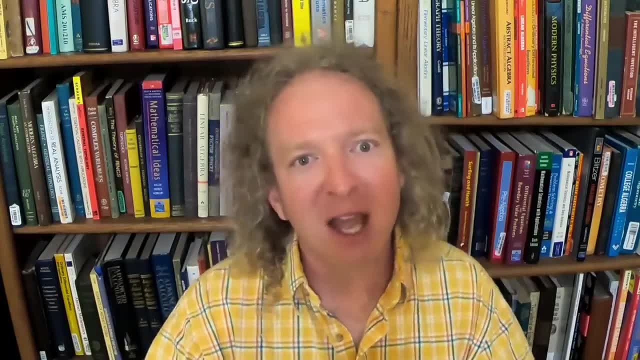 You know what that fear was. I was worried that I would run out of time. That was my biggest fear. I'm going to take the test. I'm going to run out of time. I'm like teacher's: going to take the test. 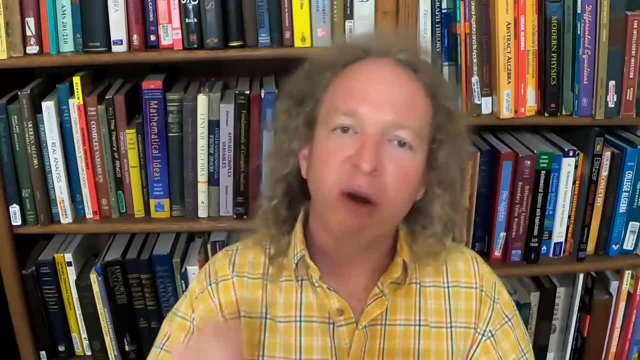 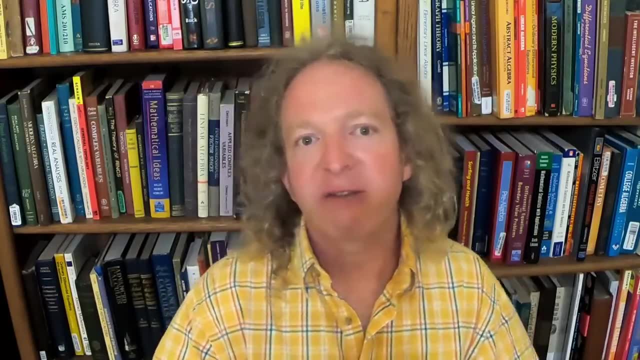 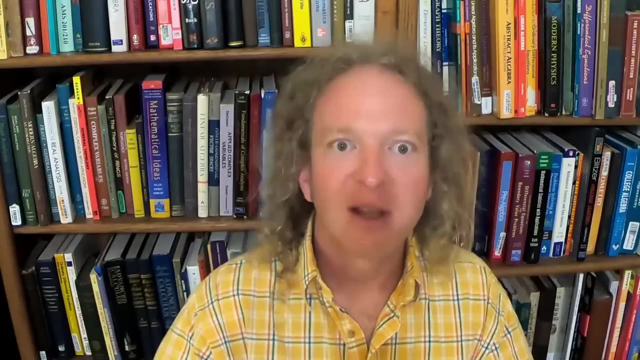 And what am I going to do? Speed. So work on speed, Speed. Not only does speed let you finish the test, there is a weird second benefit of speed: It's that it lets you redo the test. That's right, You can take a test and redo it. 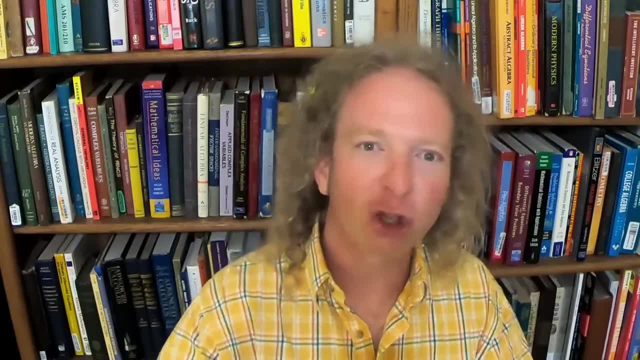 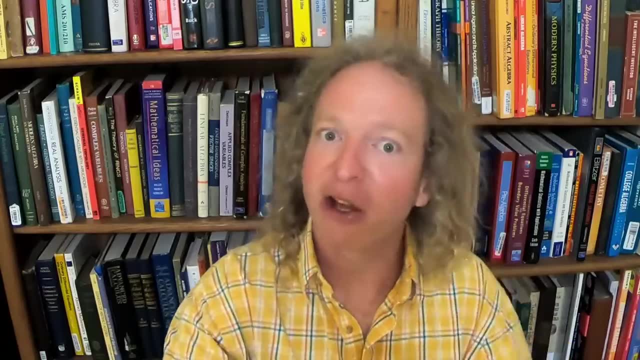 So you get to the point where you're so good, you're so ready that you take the test. you finish the test and then you do it again. That's right, You actually do it again, Not look it over, You just do it again. 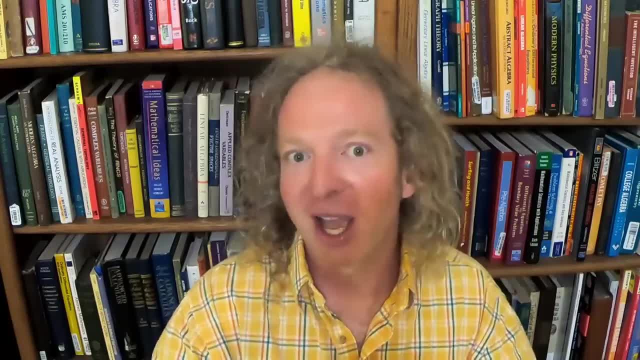 And then you compare your answers. Right, There's a difference between looking over your work and redoing it. Right, You're redoing your work, Just like if you're a programmer. you know there's a difference between looking at someone. 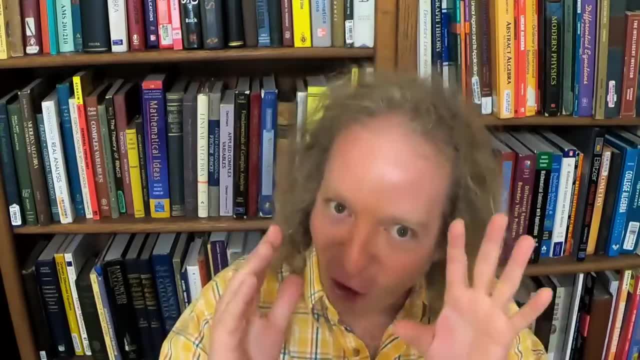 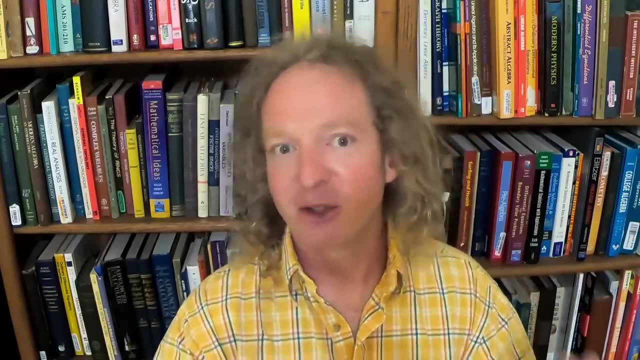 else's code and writing your own code. It's harder to find mistakes if you're just looking at your work, But when you're redoing your work you're less likely to make the same mistake. So speed. So that's my advice. 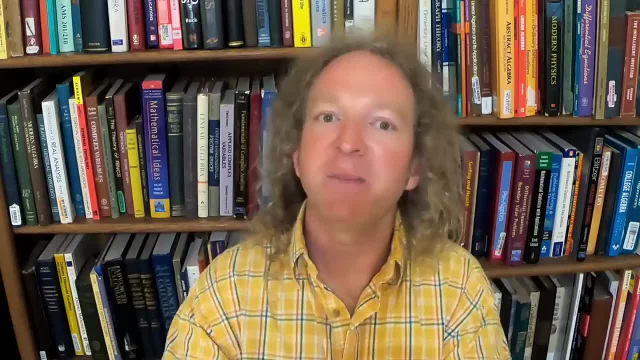 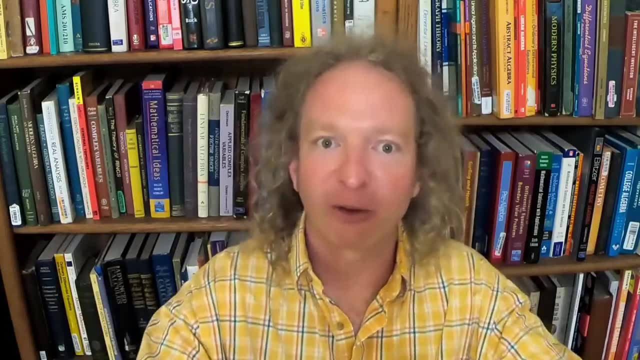 Speed, Work on speed, And by working on speed, you're actually working on everything right, Because to even get to the point where you can be super fast and super awesome by doing all of your homework quickly and correctly, that means you're awesome. 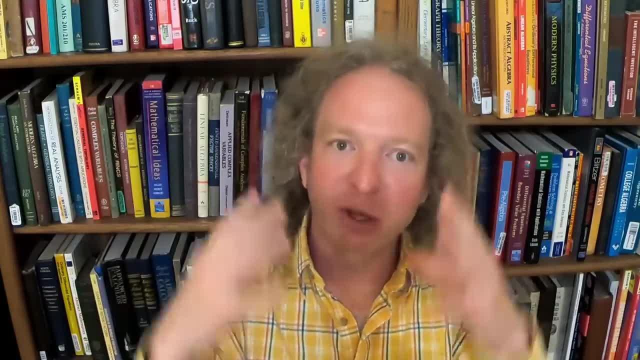 That means you're ready for the test. I mean, if you get to the point where you can work on speed, you're going to get A's and B's in most of your classes. So try it, Try working on speed, And what do you think? 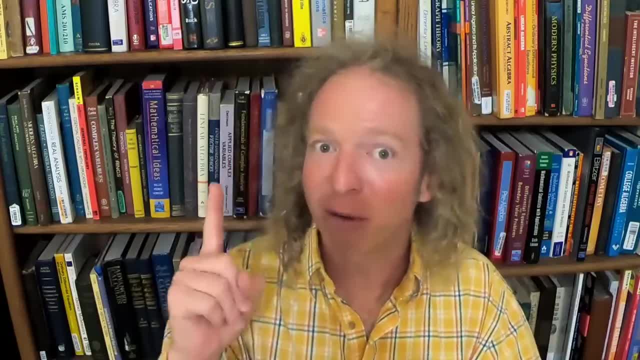 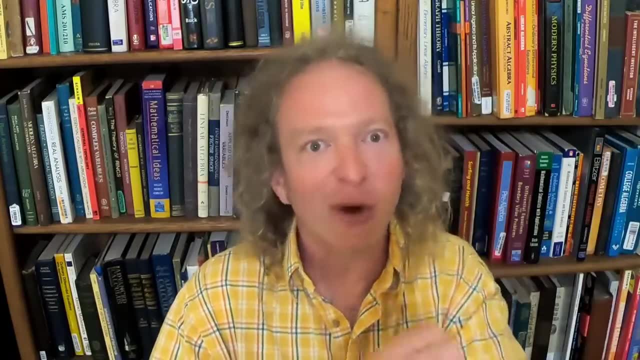 Do you work on speed? Because I actually only know one other person like in my regular life. I know one other person who told me this maybe about a year ago, that she said she works on speed And I'm like she works on, like doing the problems fast. 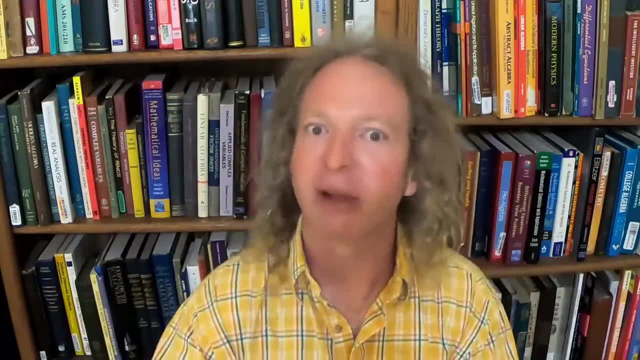 I'm like, wow, I did that too. That is so awesome, Like I'm not the only one who works on speed. So let me know, Let me know what you think. Good luck. 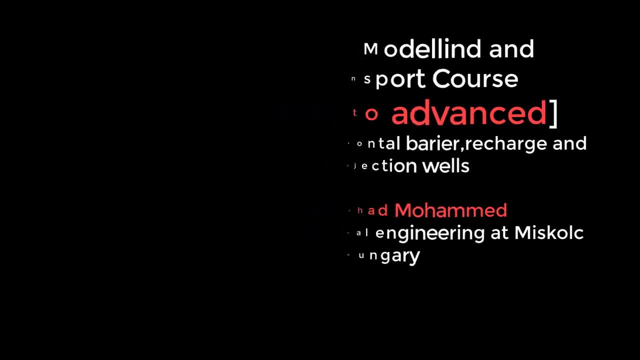 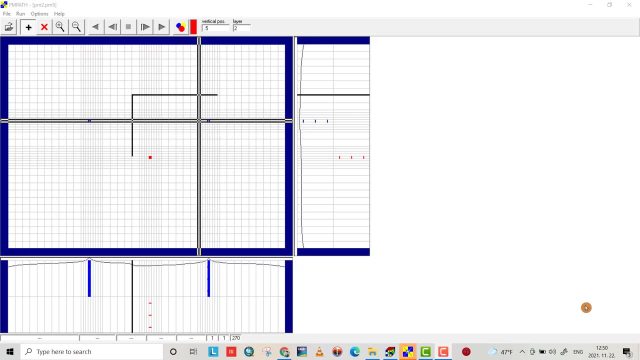 Hello friends, this tutorial is the first tutorial from the course of groundwater flow and contaminant transport. At the end of this tutorial, you can create a model which includes recharge and also two injection wells, with a production well in different levels and a barrier, as you see. 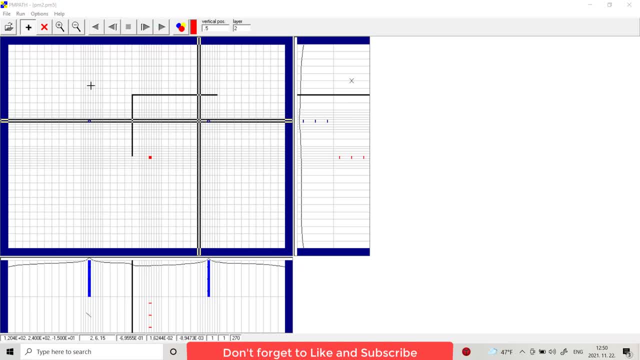 Also, you can provide particles and see how they travel from injection well to production and from production well to injection. as you see, That is the path if particles goes from injection well to the production well, As you see, I provide production well in the second layer.